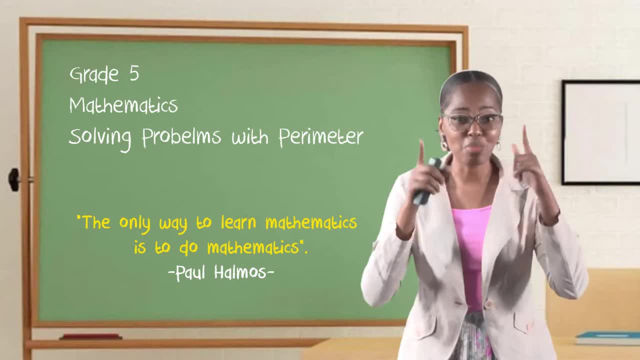 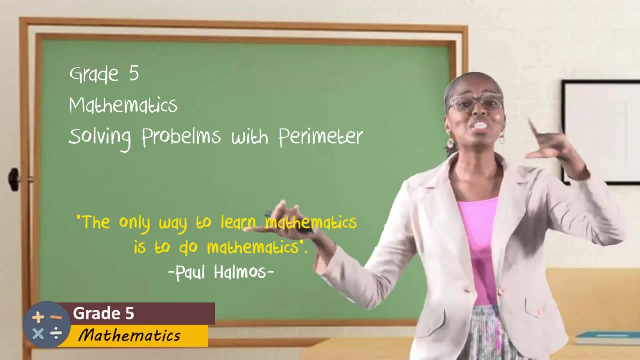 And while I'm singing, I would like for you to stand. That means get up from the chair. get up, stand on your feet and let's do some action. Every time I say perimeter is around, we're going to spin. So whenever you hear me say perimeter is around, 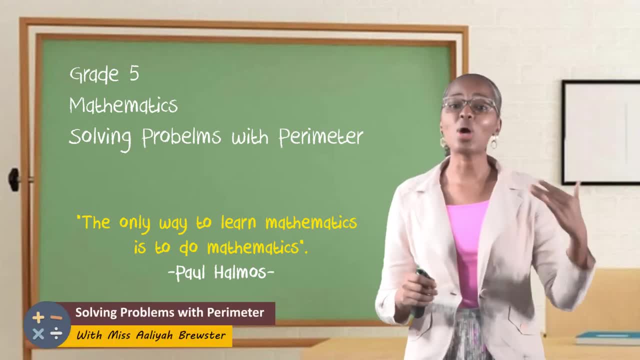 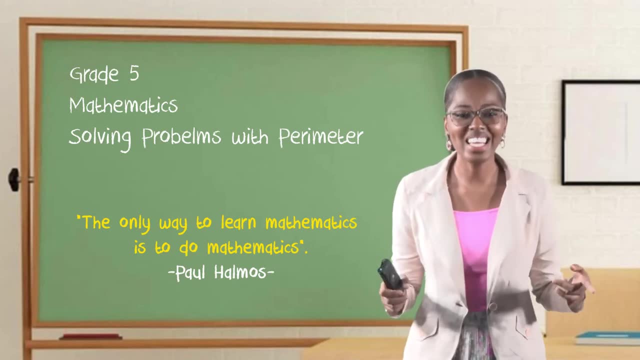 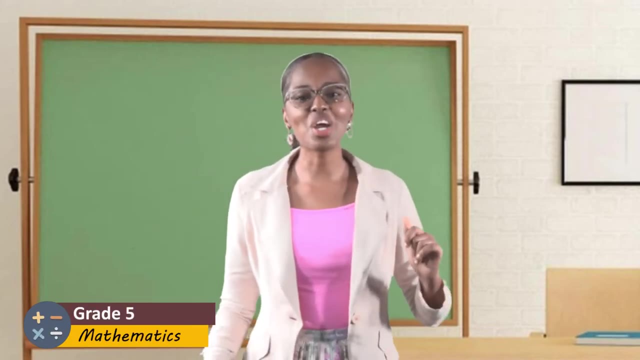 you spin one time And then I'll say something like: you add up all the sides. When I do sing that, you move your hands like this and you add all the sides. Are you ready? Let's begin. Perimeter is around. Did you spin? All right, let's try it one more time. 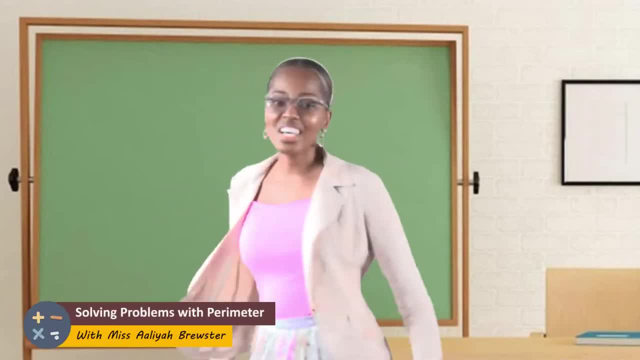 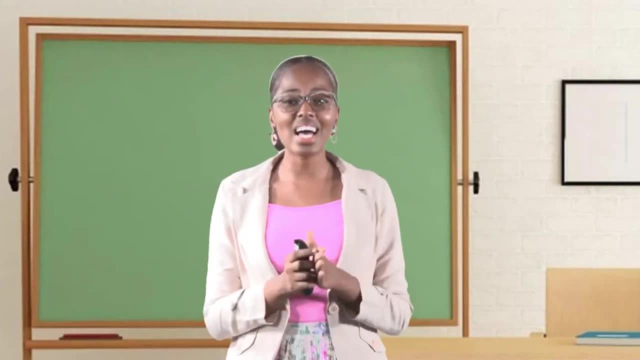 Perimeter is around. Perimeter is around. Oh, oh, don't you know. perimeter is around. You add up all the sides. You add up all the sides. Oh, oh, don't you know. You add up all the sides. 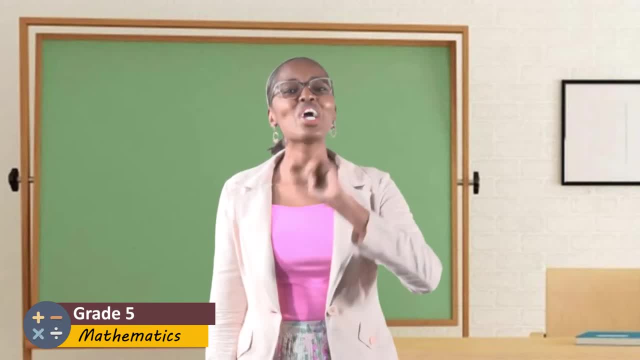 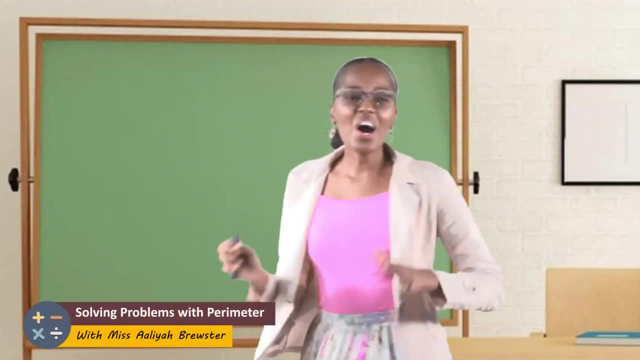 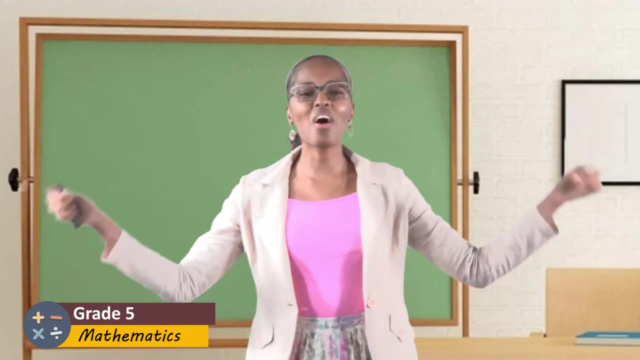 Were you ready? Did you understand? All right, let's try it one more time. Let's go. Perimeter is around, Perimeter is around. Oh, oh, don't you know? Perimeter is around. You add up all the sides. You add up all the sides. 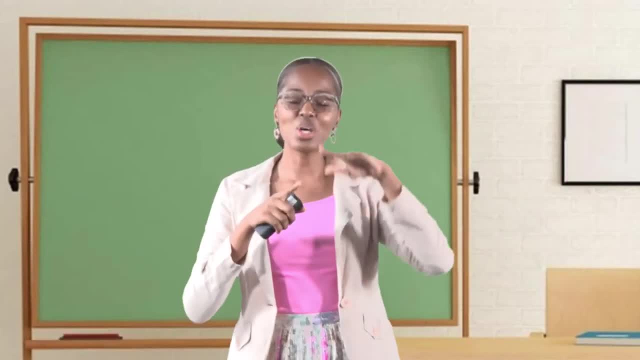 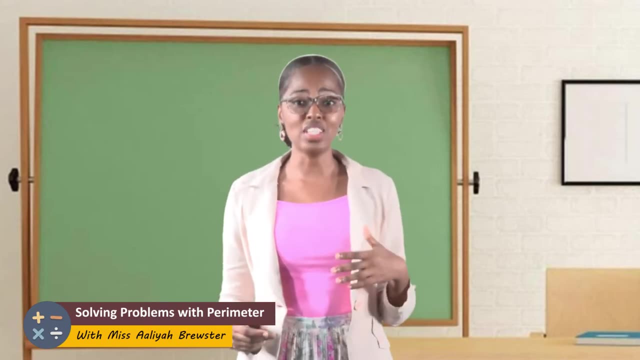 Oh, oh, don't you know? You add up all the sides. Phew, That was a workout in itself. Let's do it again. right, All right. now that you're all warmed up, it's time for us to dive into our lesson. 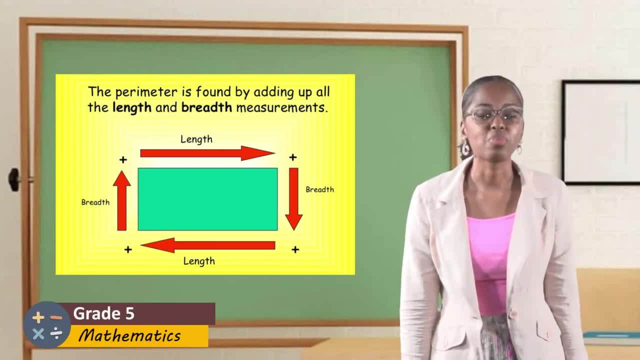 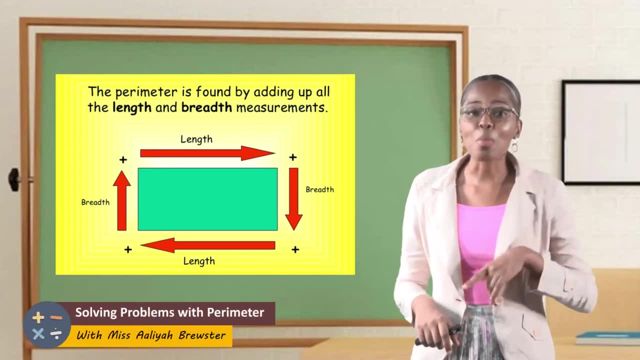 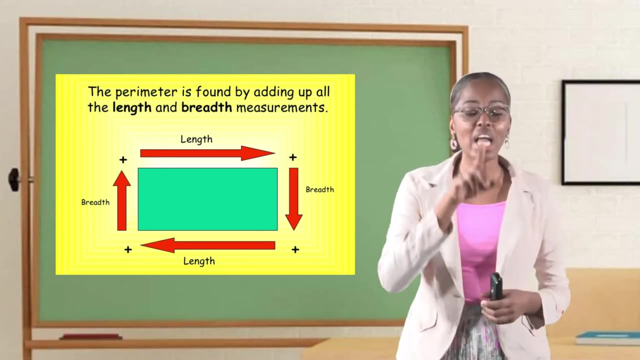 So again we're going to recap what is parameter. Parameter is the distance around a shape. Remember what the song says: parameter is around. parameter is around right. And to calculate parameter we add up all the sides. That means we add the length and the breadth. However, in some cases, 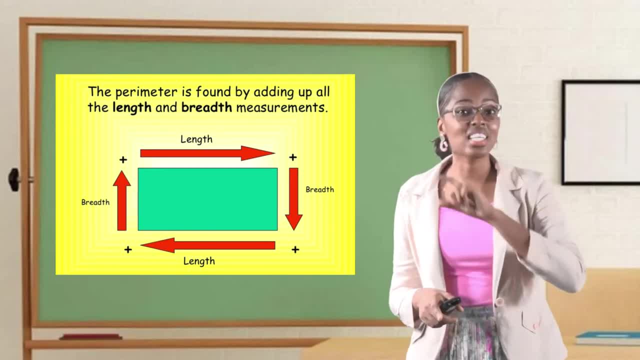 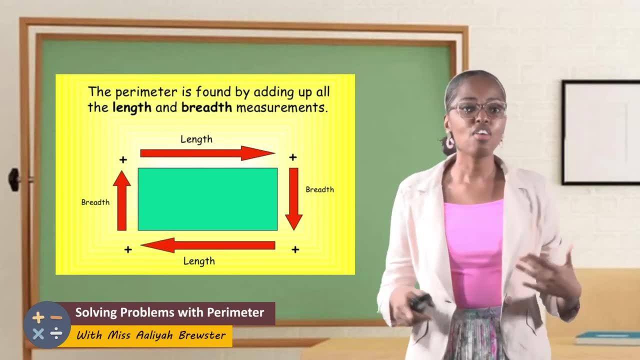 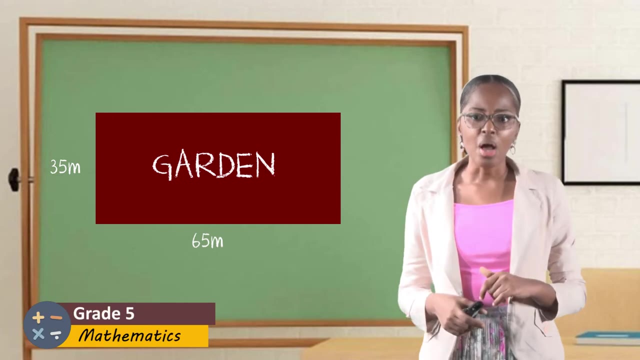 you may not be given the shape and asked to calculate the parameter of the sides. Sometimes the question can come in the form of a problem solving. For example, suppose your family has a rectangular shaped vegetable garden. Mother asks you to measure the distance around the garden. 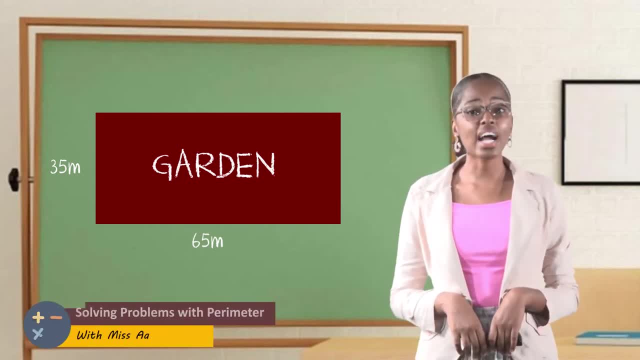 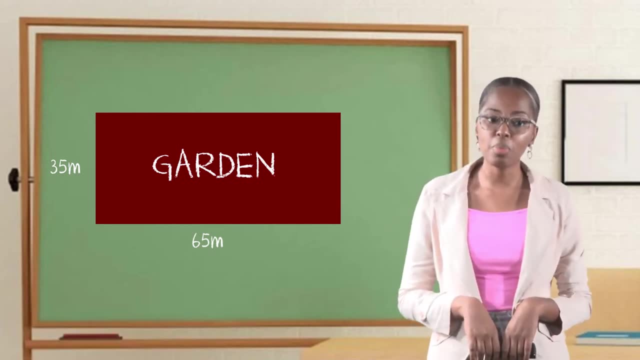 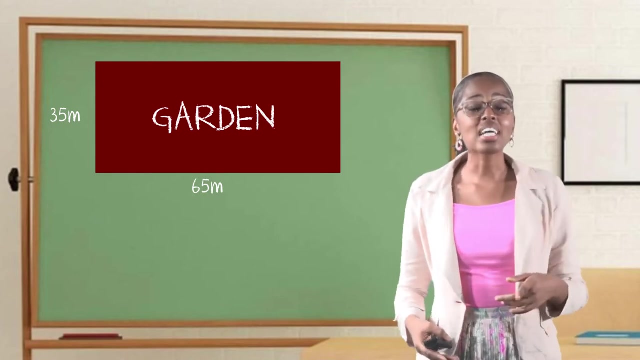 At first you were uncertain and didn't know where to start, but then you remembered that parameter is used to measure the distance around Using a measuring tape. you measure the length, that is 65 meter, Then you measure the width, which is 35 meter. Therefore, what is the parameter? So, in this scenario, you were asked: 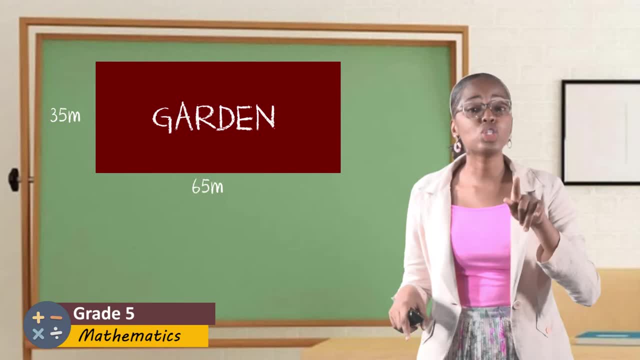 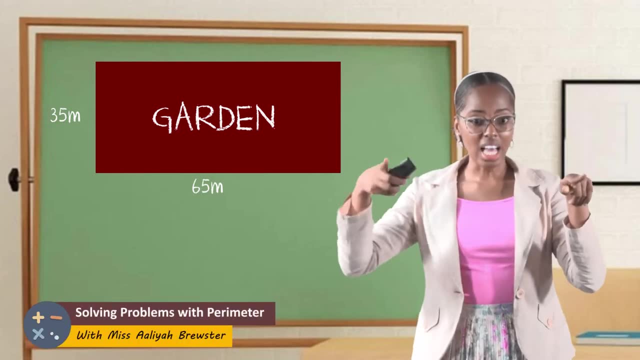 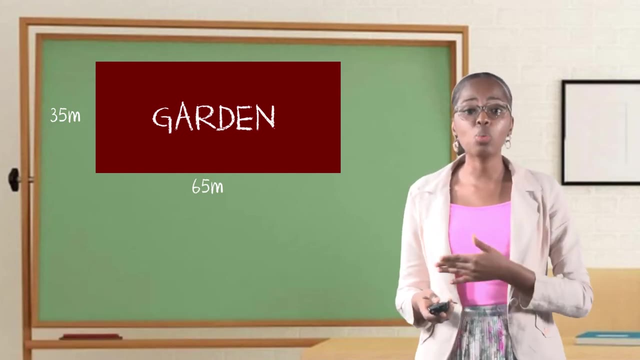 to measure the shape of a vegetable garden And from the question we know that that garden is shaped like a rectangle. However, we were given the length and the width, the length being 65 meter to the width. Since we are given the length and the width, we can assume that the two sides of the 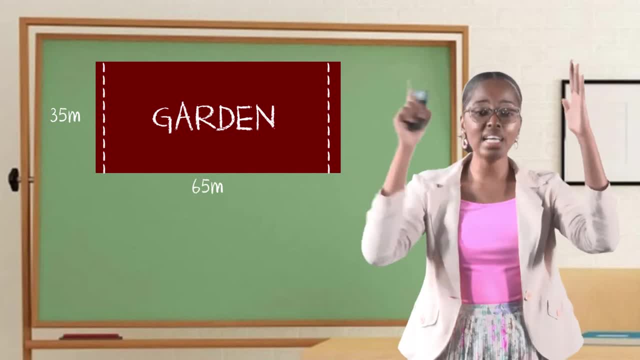 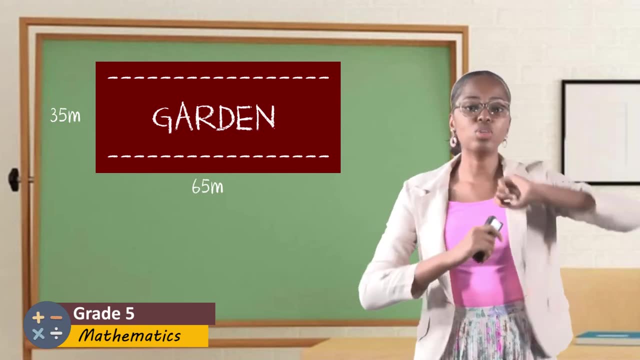 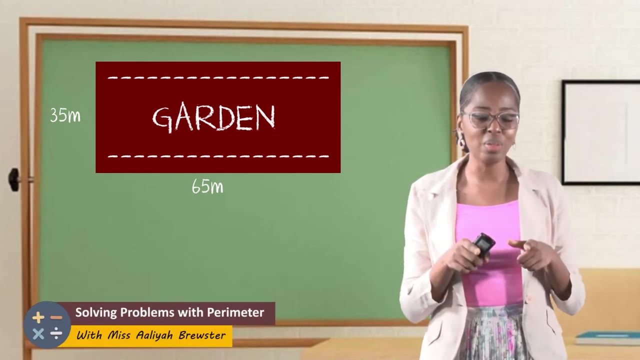 rectangle, which would be the width, both sides are measured at 35 meter and the two sides that run horizontally, both of those sides are measured 65 meter. So to calculate for the garden or the parameter for the garden, we can use the formula method, which is parameter equal to two times length. 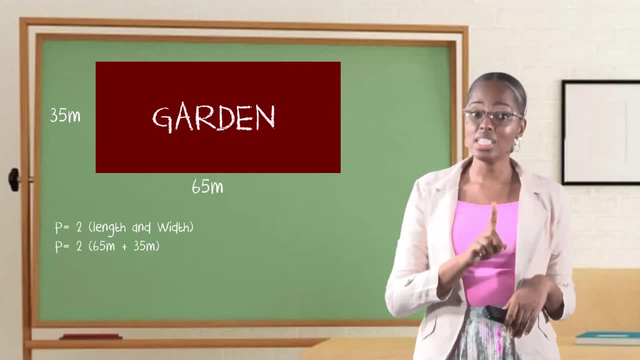 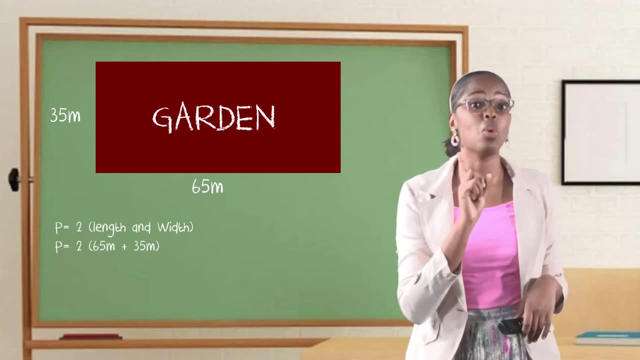 and weight, And that would be 2 times 65 meter plus 35 meter, And that would be 2 times. if we add 65 and 35, that would give us 100.. So that would be 2 times 100, which would give us of. 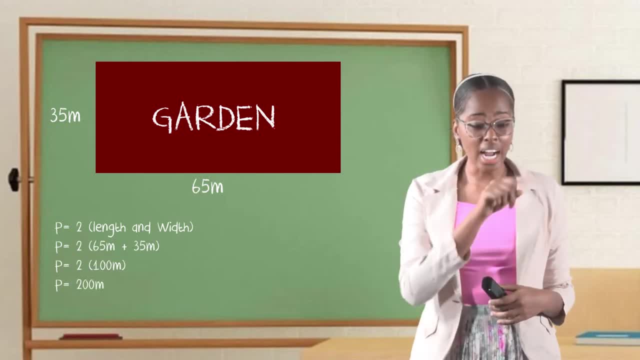 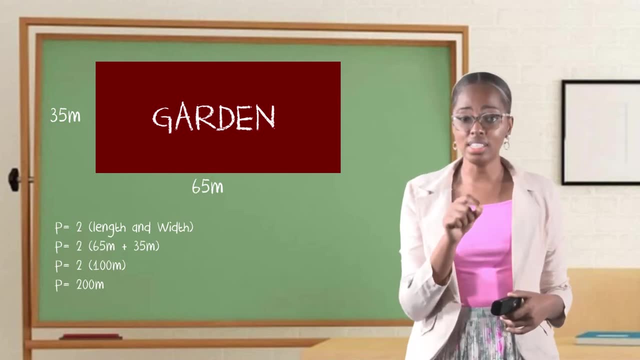 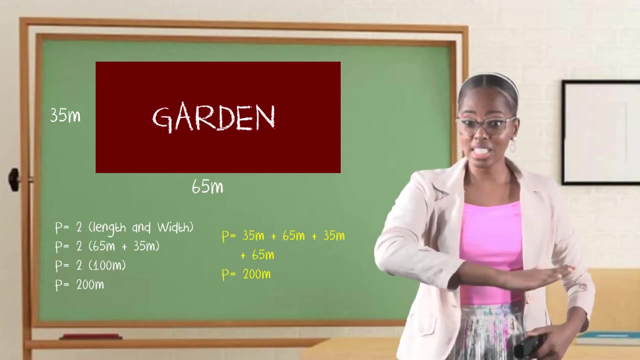 course 200.. Therefore, the perimeter for the garden would be 200 meter. We can also solve it another way by simply adding all the sides together. So we add 35 meter plus 65 meter, plus 35 meter plus 65 meter, And that would give us 200 meter. So whether you work in the formula, 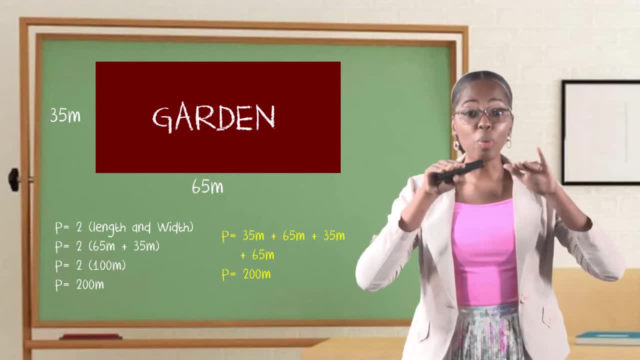 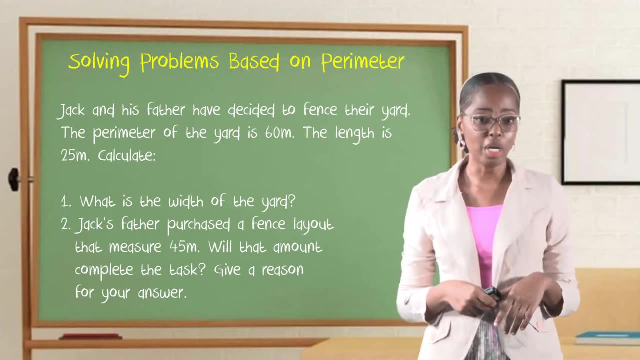 method, or you add all the sides, you're supposed to get the same answer. Let's do another example to better understand how to solve problems based on perimeter. For example, Jack and his father have decided to fence their yard. The perimeter of the yard is 60 meter and the length is 25 meter. 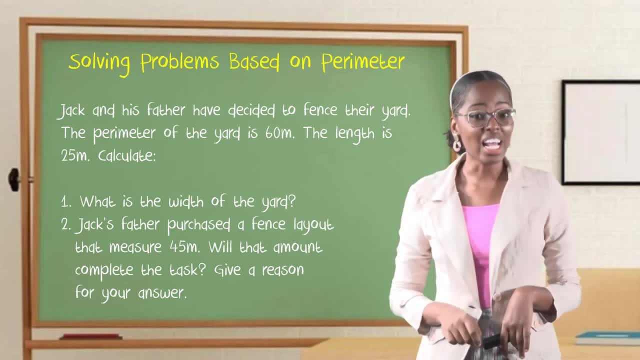 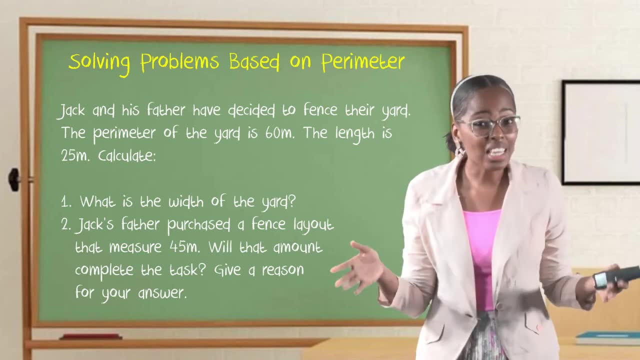 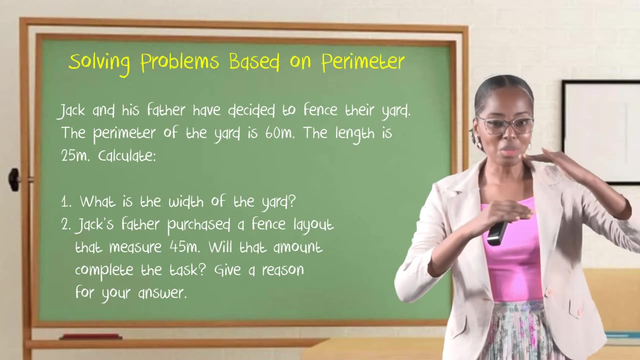 Calculate: 1. What is the width of the yard? And 2. Suppose Jack's father purchased a fence layout that is 45 meter. Will that amount complete the task? Give reason for your answer. To solve this problem, we're going to dissect it piece by piece, All right. So from this scenario we know that the 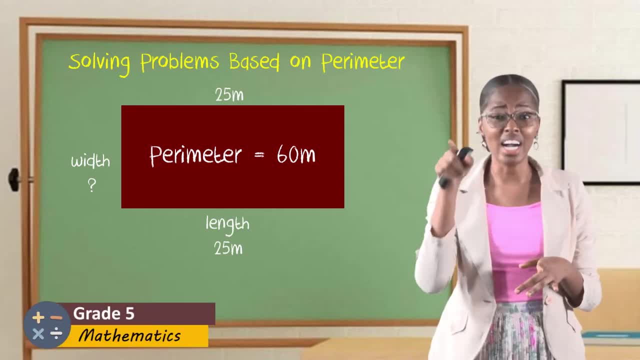 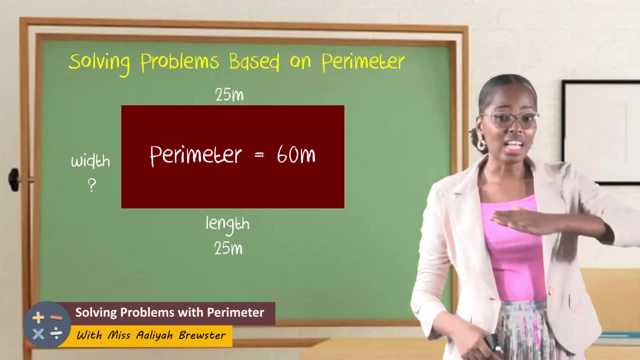 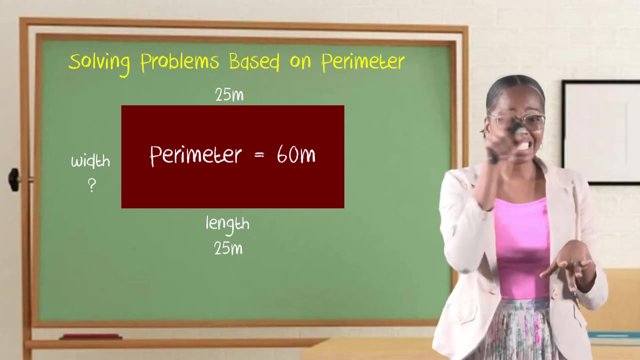 perimeter, which is the distance around that entire yard, is 60 meter, And we also know that the width is 25 meter, meaning that the length this way and the length this way would be 25 meter. However, the distance around the entire shape is 60 meter. With that knowledge, we can calculate the. 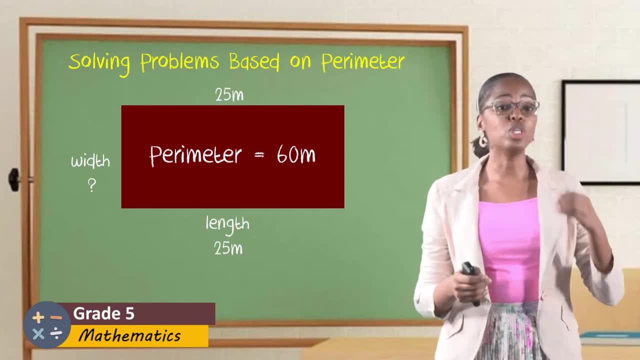 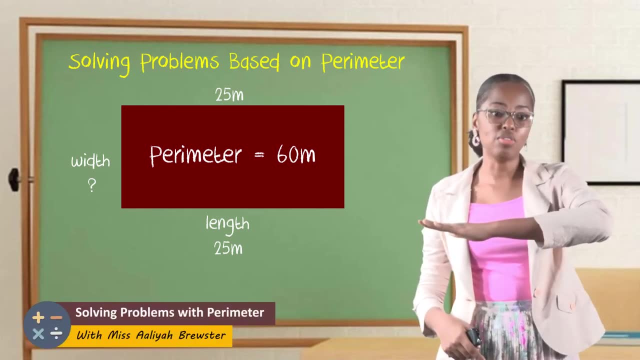 width. Let me show you how. First we add up the total length, So we add up the length that we were given, So we know that one part of the yard is 25 meter and the other part is 25 meter as well When 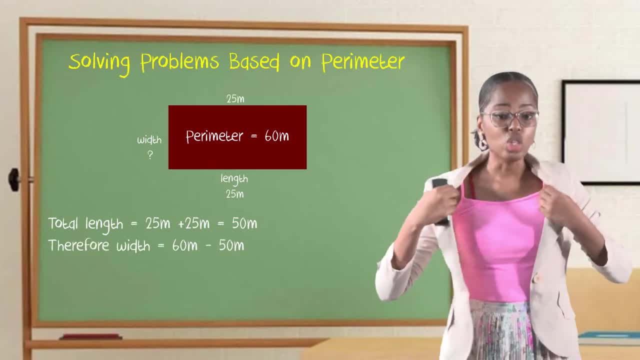 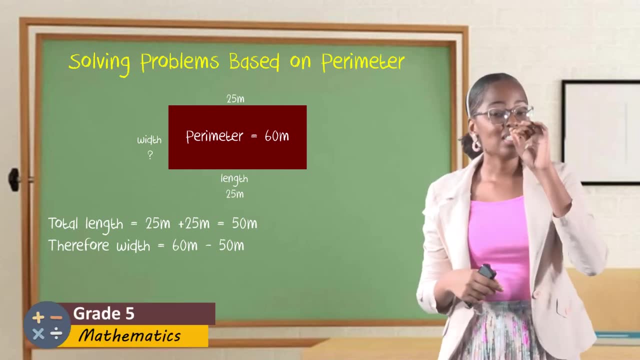 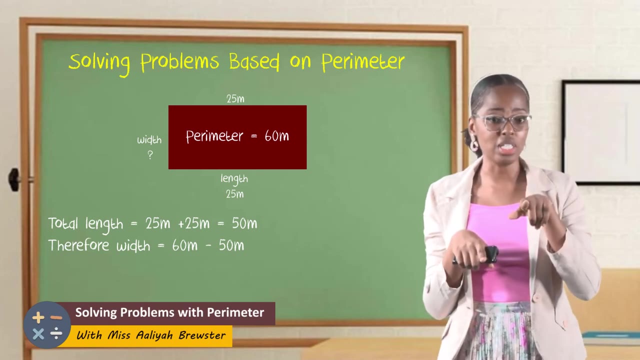 we add the length together, we'll get 50. Therefore, the width would be 60 meter minus 50 meter. All right, So we're taking away the two lengths that we know about from the overall measurement of the yard, which is 60 meter. When we subtract those two, we get 10 meter. So 10 meter is actually. 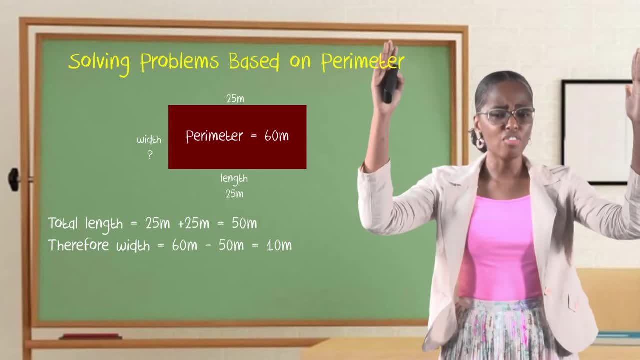 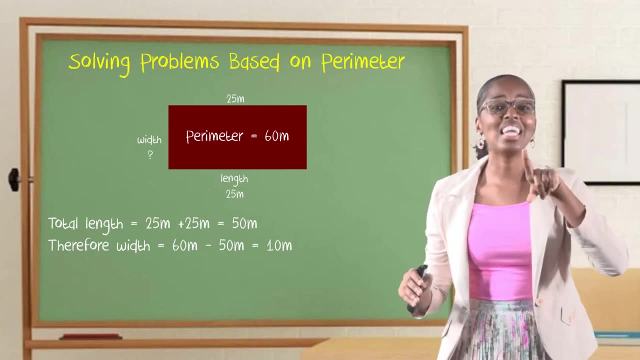 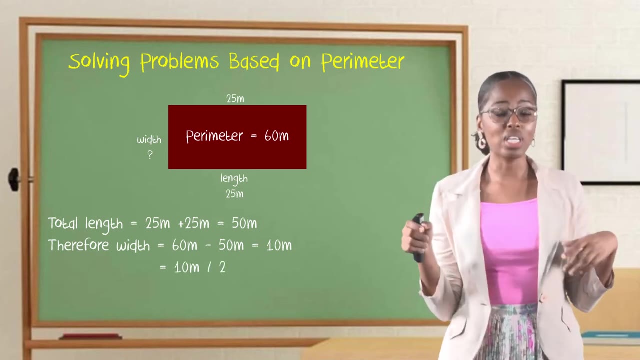 the measurement for these two sides of the yard, or in other words the width. However, it does not stop there, Remember, we're asked to find the length of the width, one width right. So we take that 10 and we divide it by two, and that would give us five meter. Therefore, the width of 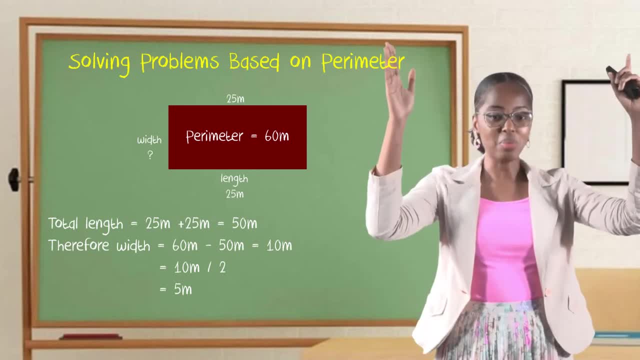 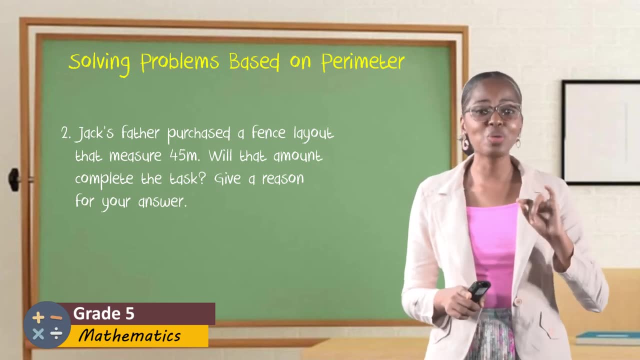 that shape would be five meter and five meter Boys and girls. we're not finished here. Remember the second part of the question. We were tasked to do, another problem solving. Suppose Jack father purchased a house. We're going to buy a house. We're going to buy a house. We're going to buy a house.